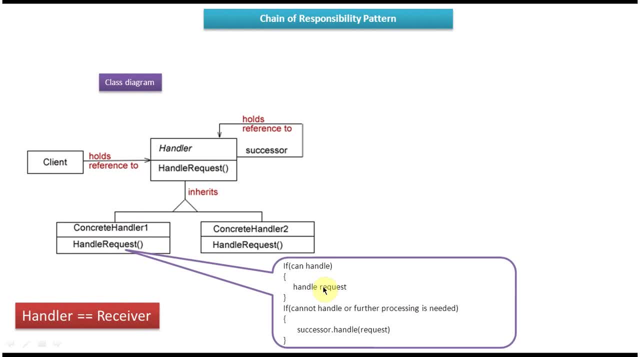 Then it will handle the request. then it will check further processing for that particular request is needed or not. if it is needed, then it will pass it to the next handler in the chain. Suppose say, when request comes to this concrete handler, if it cannot handle, then it will pass the request to the next handler in the chain. okay, that's what it is mentioned here. if it can handle, it will handle the request. if it cannot handle, or further processing. 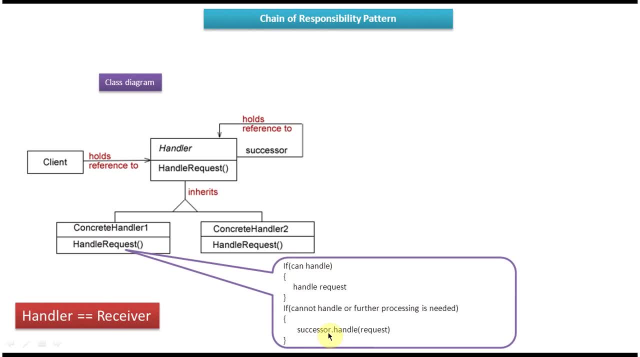 Okay, so that's what hold request or the request S transferring is needed. then it will pass it to the next handler in the chain. okay, and we will see the key sequence diagram next. So here we can see cilind and handler. handler 1, handler 2: this is the first handler in the chain and this is second handler in the chain. so client send request to the handler. 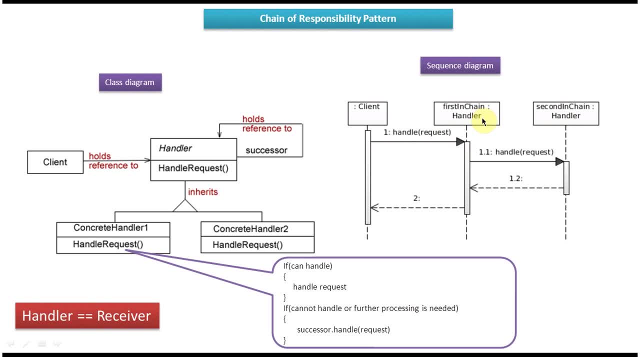 saying: please handle this request. So this handler will check whether his request is rejected, it can handle the request or not. if it can handle, it will handle the request and then it will check further processing for the request is needed or not. if it is needed, then it will send it to the next handler in the chain. okay, 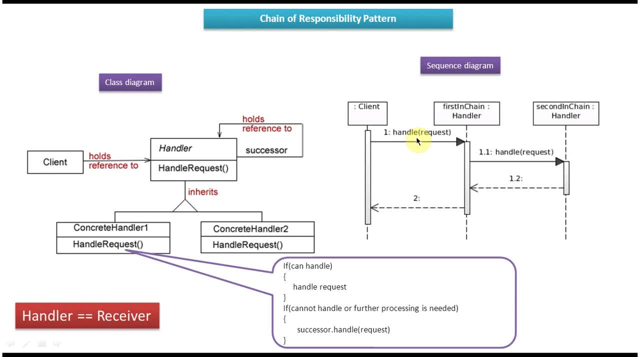 and suppose, say, client send request to the handler saying: handle this request. if, if the, if this handler cannot handle the request, then it will just pass the the request to the next handler in the chain and next handler will check whether it can process the request or not. if it can handle it will handle, otherwise it will pass. 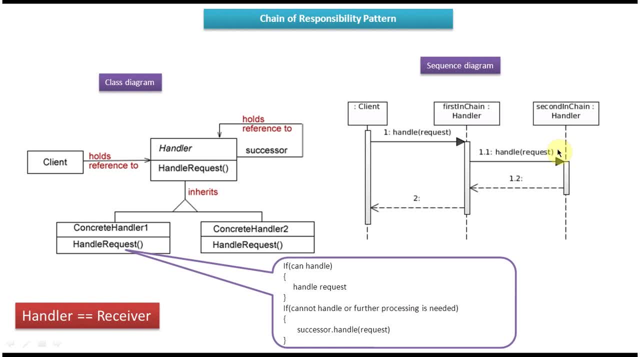 to the next handler in the chain until request is processed by the handler. like that, the request will pass to the next handlers. okay, and this is about class diagram and sequence diagram of a chain of responsibility design pattern. i have created separate video for chain of responsibility design button implementation where i have explained java code related to 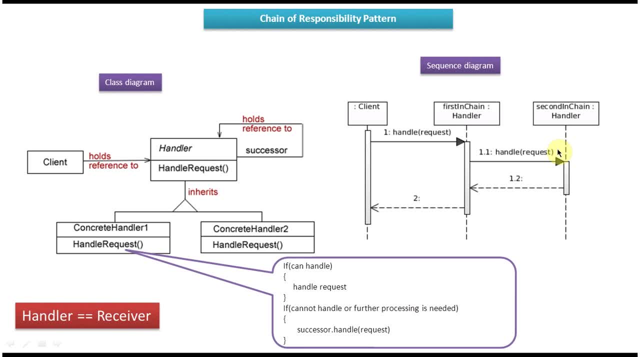 this chain of responsibility design pattern and this is about chain of responsibility design button, class diagram and sequence diagram. and thanks for watching. bye.